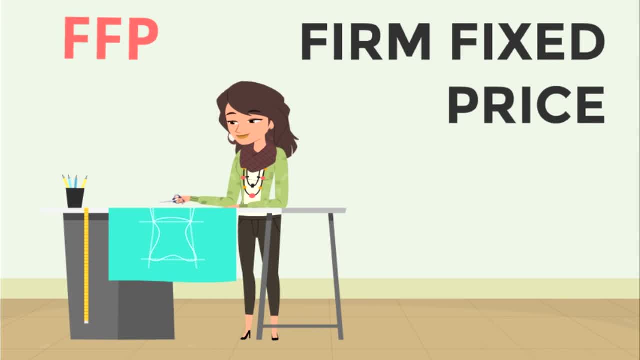 was fixed and you didn't need to pay anything else, You probably would go for the FFP And the firm fixed price is the most favored contract type by buying organizations. People love to buy when there are no surprises. As much as possible, buyers go for the firm fixed price. 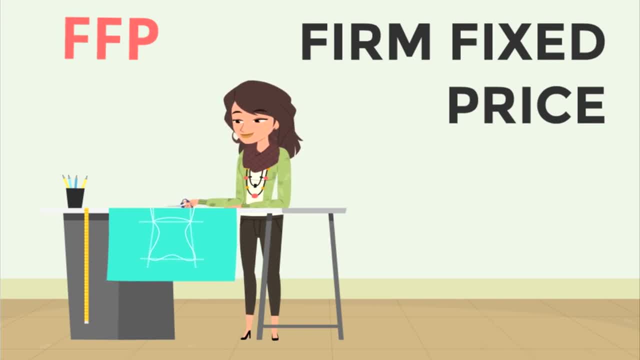 because they know there will be no changes. Now, if you decided that, in addition to a pool, you wanted a fence, then you wouldn't be surprised if there was an increase in the price, would you? And that's the thing about FFP: There could be changes if the scope changes. 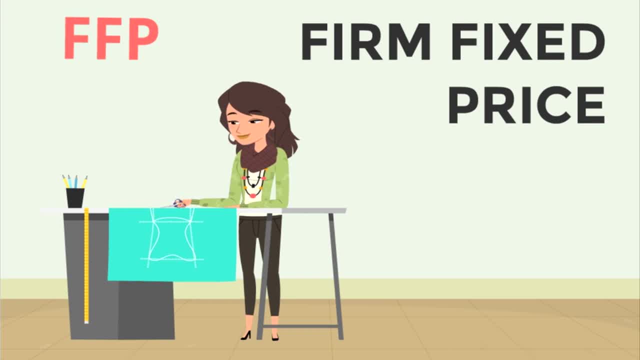 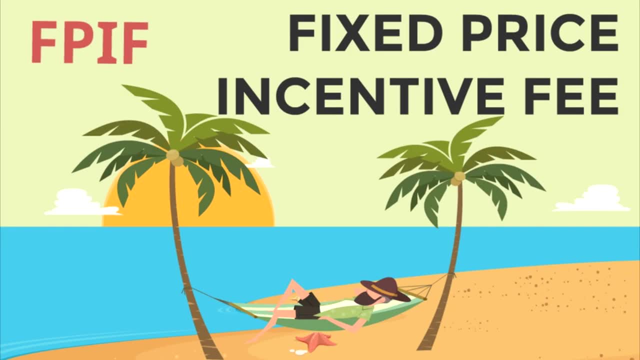 But if the scope of work doesn't change, then you don't expect to have any surprises. That's FFP. The next contract type is FPIF- Fixed Price Incentive Fee. There's an incentive to the seller. Does the seller want to take an awesome vacation on the beach? Sure. 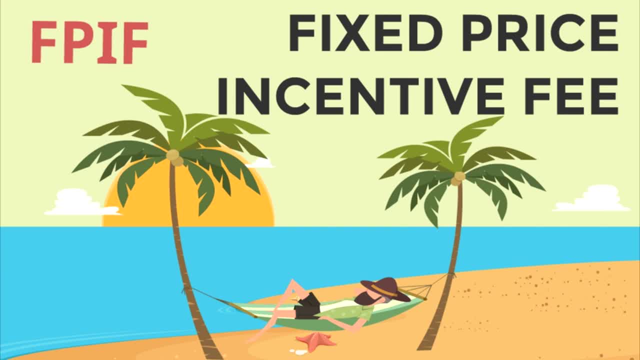 Well, they're going to have to step up their game. The Fixed Price Incentive Fee contract gives the buyer and seller some flexibility in that it allows for some deviation from performance, with financial incentives tied to achieving agreed upon metrics. If you get this project done early. 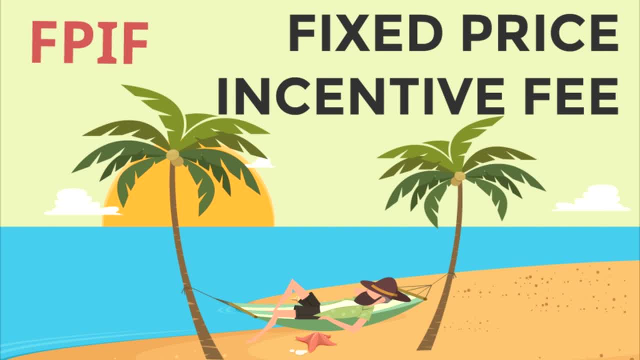 then you will get some additional incentives. But if you can get this done three weeks earlier than the expected date, then you will get some sort of incentive. Or if you can get this done to this particular quality standard, then you will get some particular incentives. So typically such financial incentives- 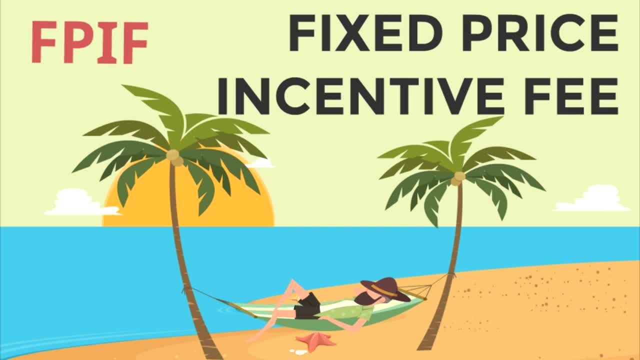 are related to cost schedule or technical performance of the seller And under the FPIF a price ceiling is set. And you 3 sabe why? because, hinters, I know there have been some good figures on first date: £28,000, bah, so usually the other. 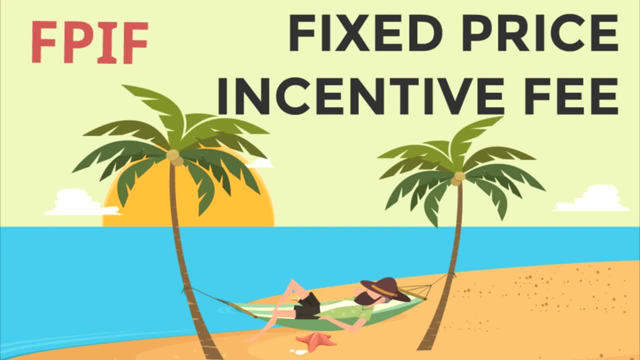 all costs above the ceiling price are the responsibility of the seller. In this contract type we typically hear the term the point of total assumption being used. but for your exam I wouldn't get carried away with the PTA. The PTA at a high level is illustrated in terms of a ceiling price above which the 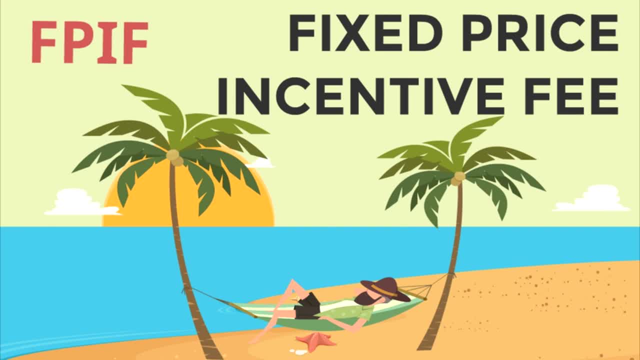 responsibility for the costs lie on the side of the seller. If the seller goes higher than the ceiling price, that's their business. Now there are various components in the FPIF contract, but those are beyond the scope of the PMP exam, in my opinion, and I don't think you need to go that far. 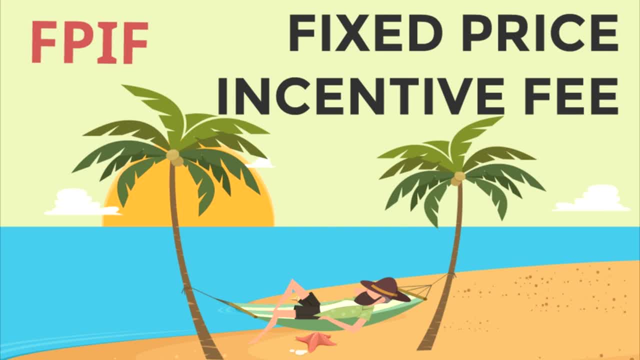 memorizing the PTA. Once upon a time we had this on our mock exams, but we found this to be a waste of time for the poor student who usually doesn't get a single question on PTA. So, as long as you understand the concept, the fixed price, incentive fee contract. 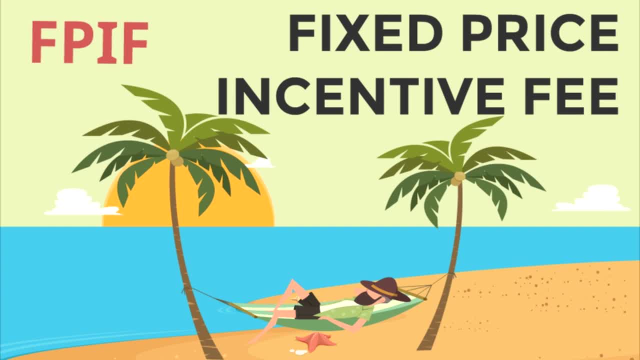 is one in which the seller has a fixed price set for what is being done, but there is the possibility of an incentive. Now, if the seller burns through their profit within that fixed price and at the same time burns through any potential to get an incentive, then at that point they 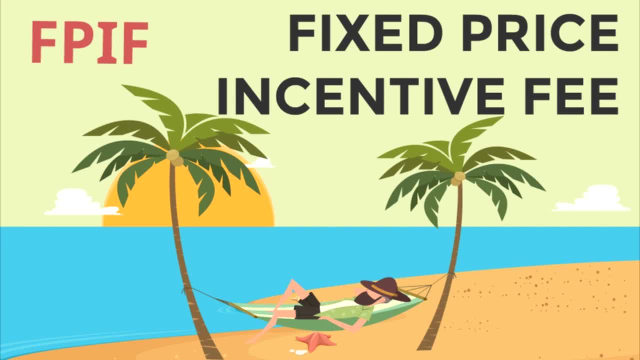 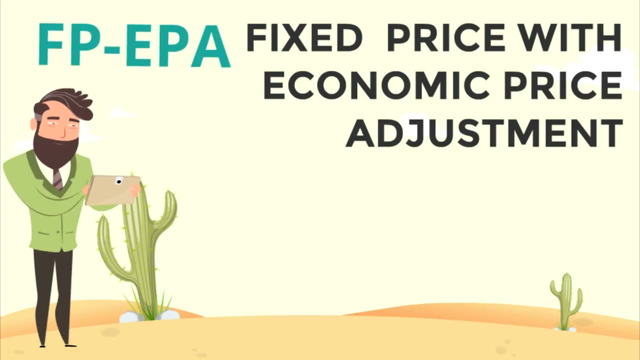 then assume all of the cost and that's why it's called a point of total assumption. but that is beyond the scope of the exam. like I said, The next contract type is FP-EPA- Fixed price with economic price adjustment, and this contract type allows. 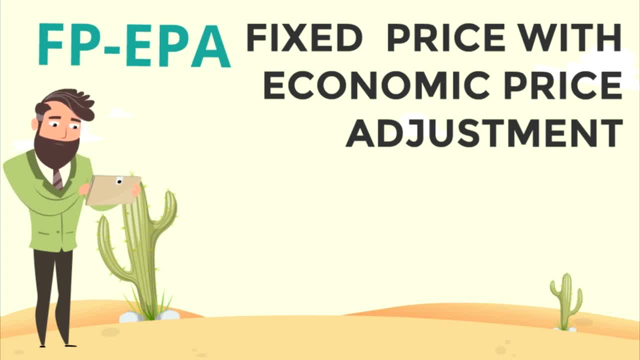 a clause for inflation. if the contract spans across several years, then it makes sense for the seller to tell the buyer: hey, because of the time value of money and the devaluation of money concept, we would like to have a clause in here for an economic price adjustment. So based on the economy, 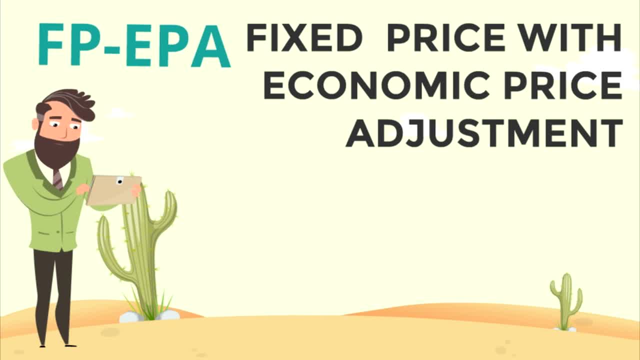 that fixed price could be reviewed Also as a result of the price of certain commodities, which could vary very widely. For example, one of my clients had a huge fluctuation in copper and copper was being stolen in the mid-2000s to late 2009-10.. 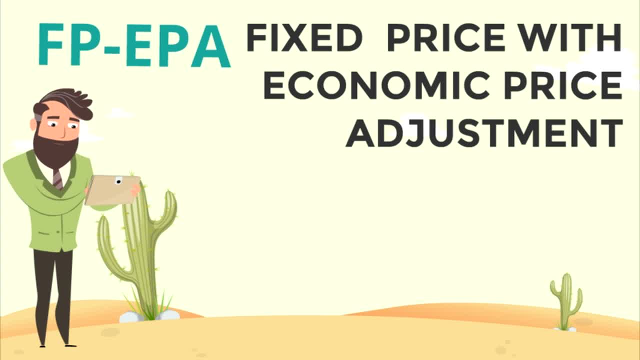 And as a result, because of the business they did with copper wiring, the prices went up quite high. That is an example of adjustment in a contract due to certain conditions or increases or decreases for certain commodities. The next contract type here is cost reimbursable. 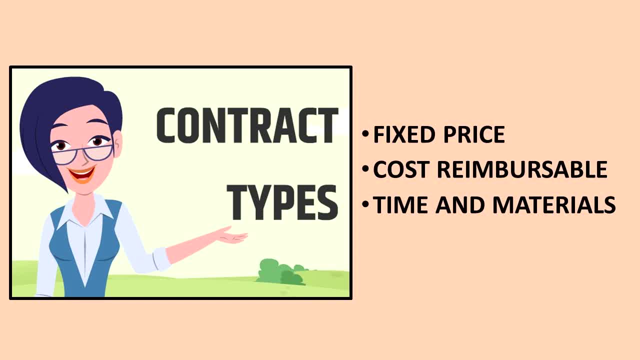 And in cost reimbursable type contracts the seller is reimbursed for all legitimate costs And that will include travel per diem where it is allowed, And for that reason receipts need to be provided in a lot of these contracts. 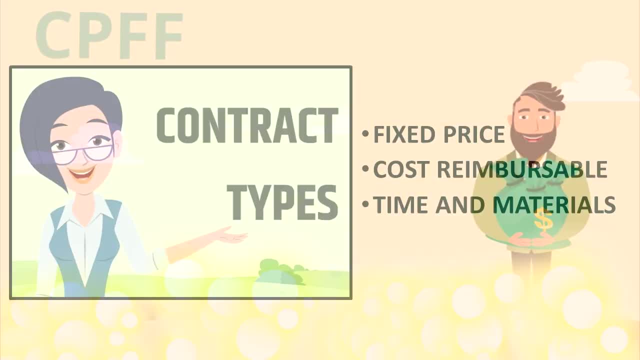 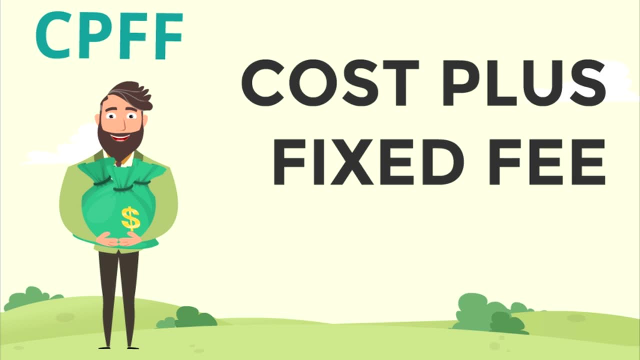 So the first one here under cost reimbursable contracts is cost plus fixed fee, CPFF. The seller is reimbursed for all allowable costs for performing the contract work. It's very straightforward: There's a fixed fee payment calculated as a percentage of initial estimated project costs. 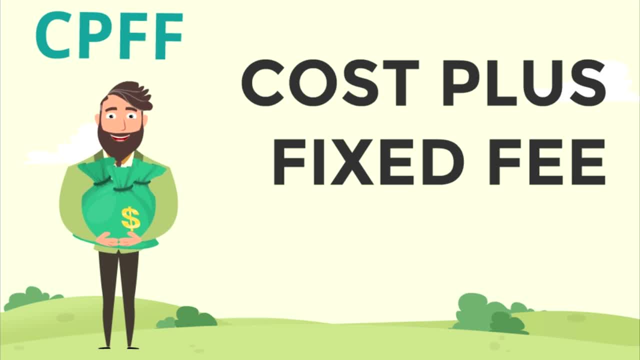 So initial estimated project cost is not the same as eventual, or at the end or in the middle, you see, And the reason is there is an illegal type of contract called cost plus percentage of costs. This contract is not it. Cost plus percentage of cost does not have the fixed fee payment calculated as a percentage of the initial estimated cost. 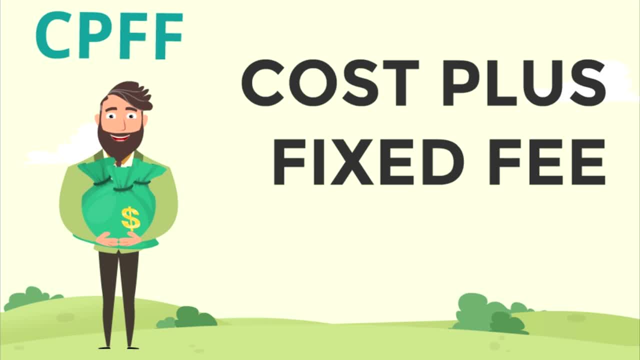 It is the cost of the project, on the other hand, a calculation based on what the total outcome is. But that's not what this is. We need to get this straight before the contract is authorized. The next contract type is cost plus incentive fee. In the same 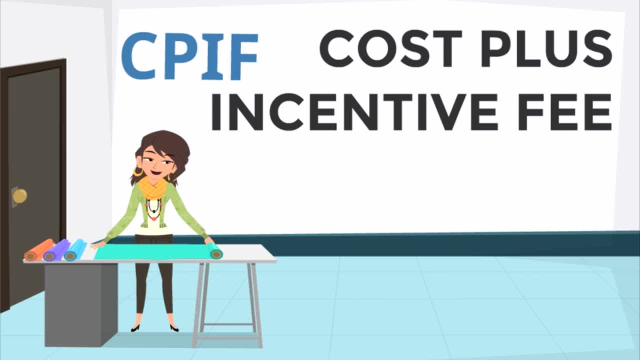 token, as FPIF, the seller is reimbursed for all allowable costs, but there is an incentive, and this incentive is similar in nature to what was discussed under FPIF, in that, based on certain performance levels- cost schedule, technical, whatever- the seller will benefit from a cost sharing formula. and 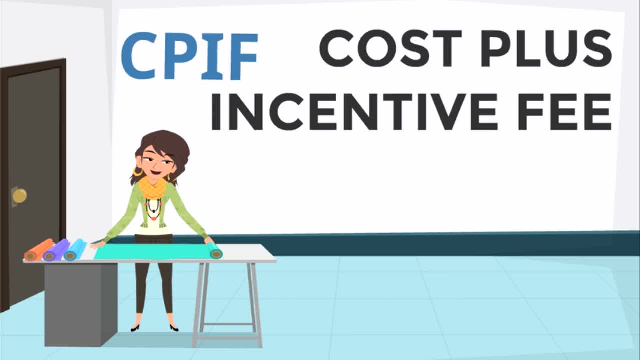 this could be an 80-20 split, a 60-40 split. it really depends on the contract. But the bottom line is: costs are reimbursed and there's an incentive on top of that. The next contract type: CPAF, cost plus award fee. the seller is. 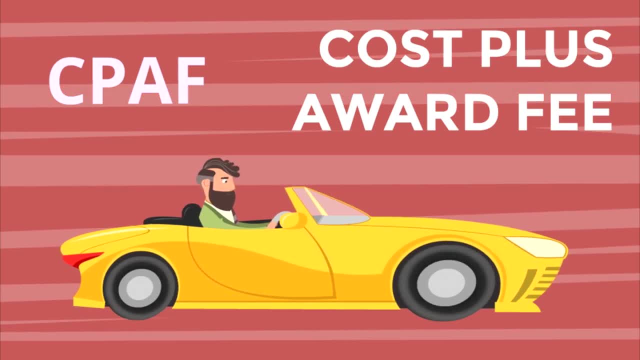 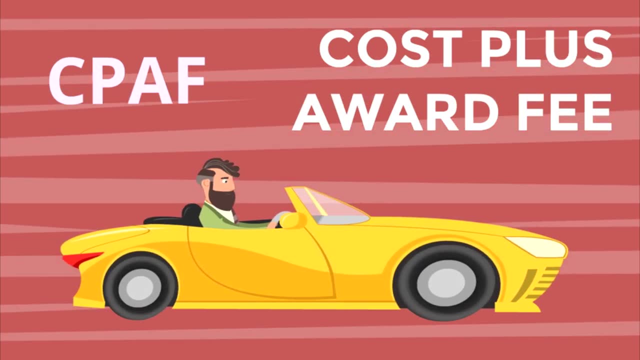 reimbursed for all legitimate costs. But majority of the fee is earned based on satisfying certain broad and subjective criteria. So there's no crying over spilled milk. You don't win the award fee too bad. The criteria is in the contract, but it's very broad and 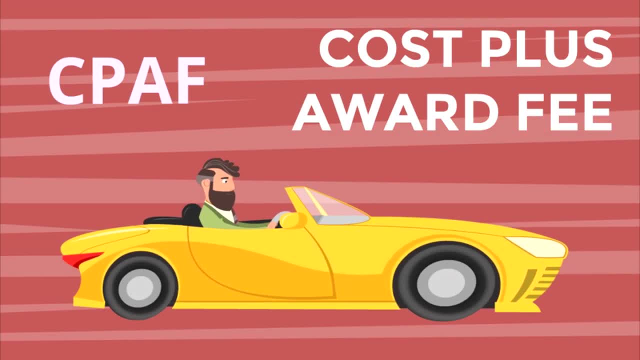 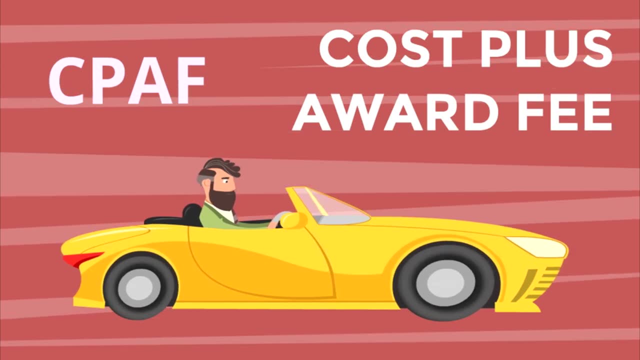 subjective. So I usually say: seller, beware, beware of who you do this contract with. Now one of our clients in the past won a massive, massive award fee as they did some business for a government and that award fee was so massive they decided to send a ton of 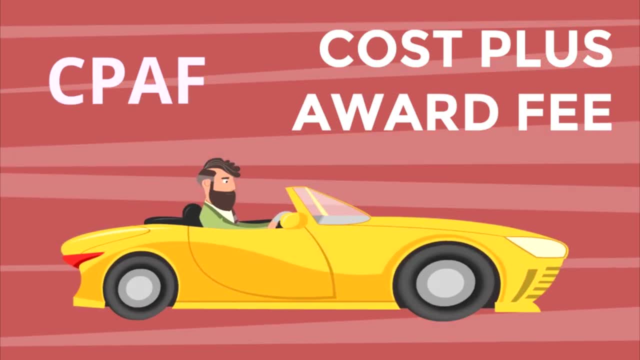 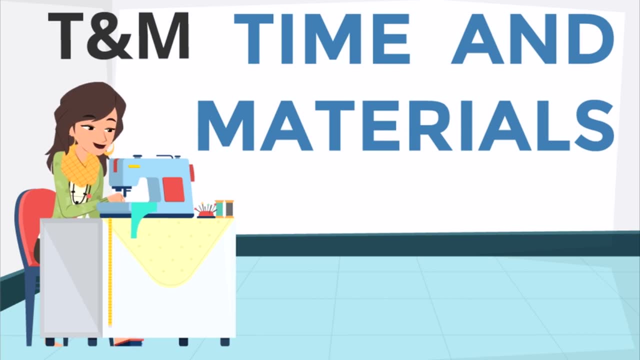 people for training with us. Of course, we were happy about that. The last contract type is T&M- time and materials contract, also called time and means, and this is a hybrid of both the cost reimbursable and the fixed price contract. They are often 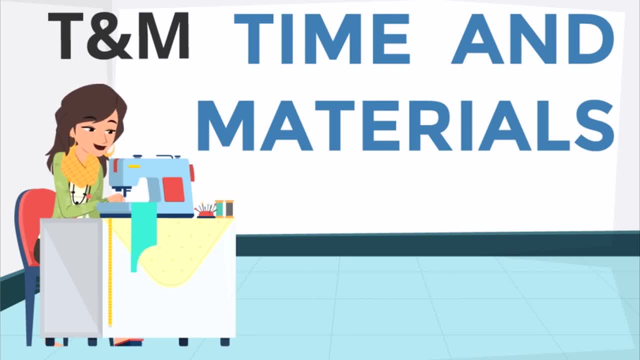 used for staff augmentation, acquisition of experts and any outside support when a precise statement of work cannot be quickly prescribed. The advantage of the time and material contract is you can go ahead and initiate the contract and you can also put a not to exceed value per time period. I worked on a T&M contract with a 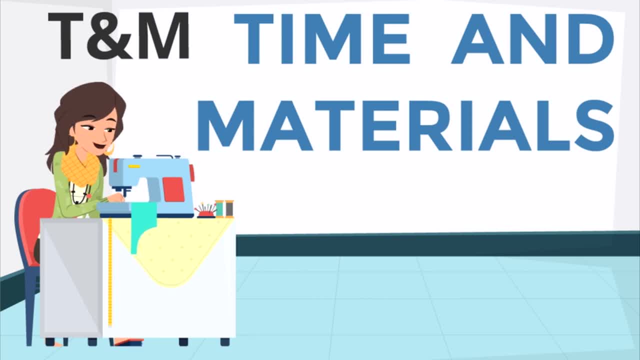 well-known semiconductor firm and they said: Phil, your project management activities need to stop at this point. You cannot go over this value. If you go over this value, we aren't going to pay. and that is an advantage, because they could go ahead very quickly, start a contract, And they 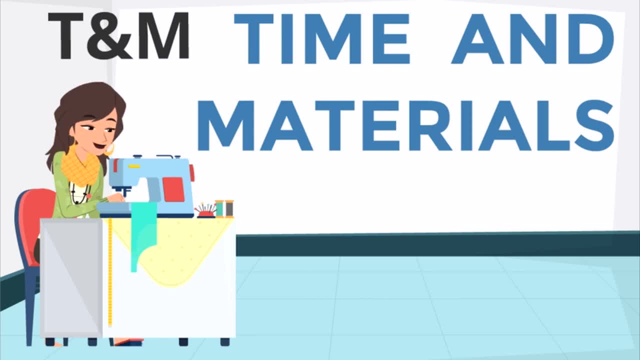 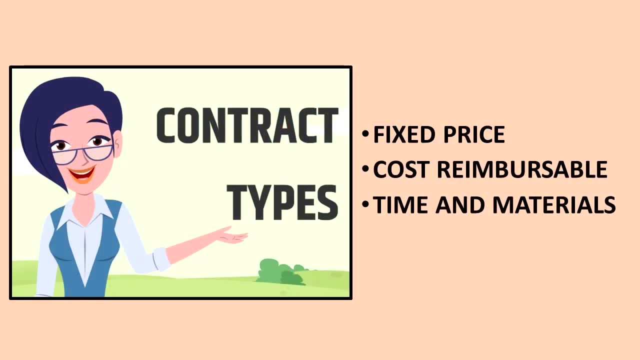 could shut it down, or the not to exceed value will kick in at any point that they're not willing to pay. So those are your three contract types: fixed price, cost reimbursable and time and materials. I hope that helped you. this is just the. 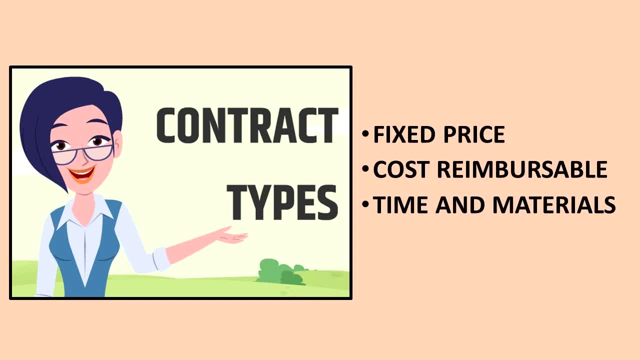 top of the waves. to get you straight Now on the exam cheap question is: which contract type is best for the buyer? So if you have FFP, FPIF and fixed price with economic price adjustment, depending on the question, the answer is most likely going to be the FFP. Now if you're painted a scenario in, 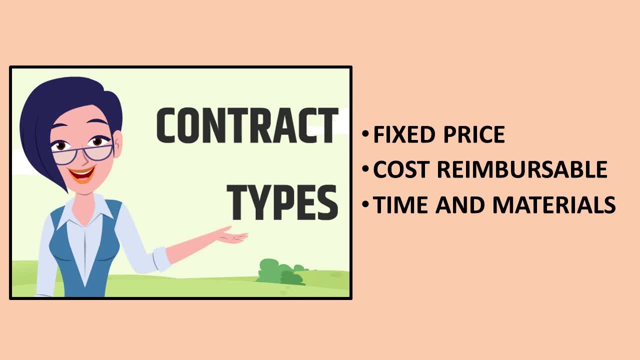 which the price of a commodity is likely to drop very, very low, and you have two options between FPIF and FP-EPA. of course you should choose FP-EPA, So the questions on the exam are going to be based on these ideas. Is an incentive necessary? Should we take the risk? 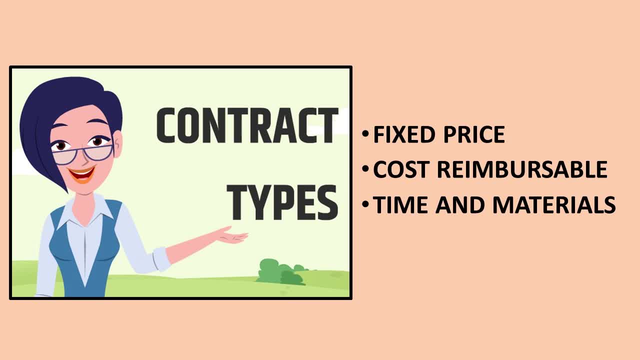 of an award fee, Do we need the cost to be reimbursed? You see, you use a cost reimbursable contract in situations where you are not totally sure of the scope of work. There is some ambiguity, There are some unknowns. 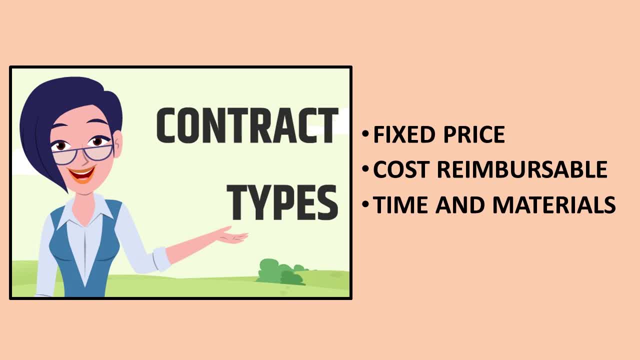 But if there are no unknowns, as a buyer you want the fixed price. Also, it is ethical to have a cost reimbursable contract if there are unknowns that could affect even the seller, because you don't want to negotiate in bad faith. So the answer is not always fixed. 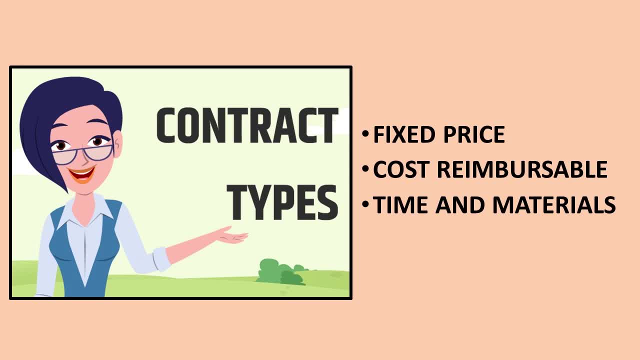 price. contrary to what a lot of trainers say Out there on social media space, sometimes a fixed price contract may not be the most ethical contract type, especially when you know there are so many unknowns, there are so many factors and you don't want the seller to be bitten in a bad way. That's called negotiating. 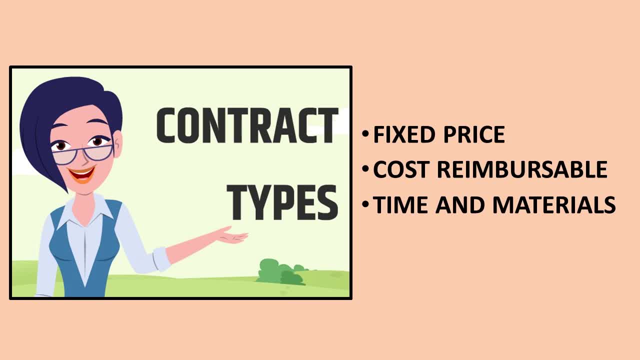 in good faith and you don't want the seller to be bitten. period: Good faith, bad faith. But anyway, that is pretty much the end of the story. I will revisit this Some other time and I hope you found some value from my rather quick presentation.